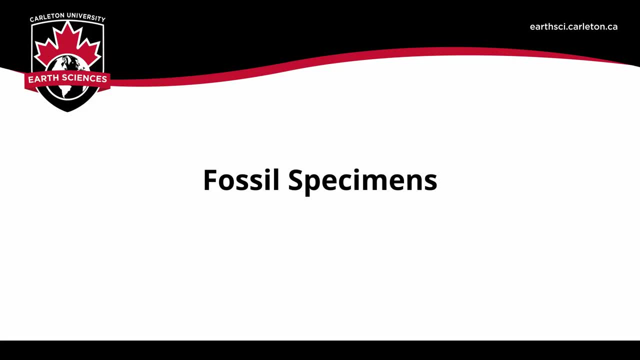 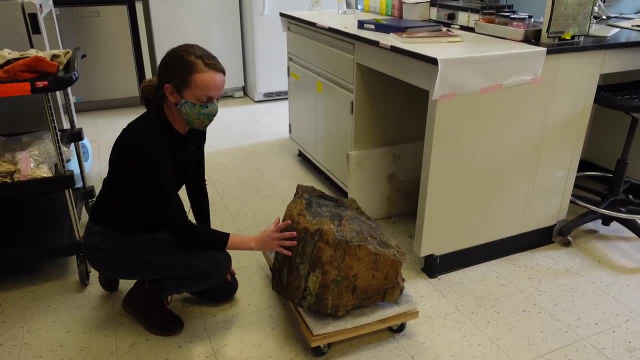 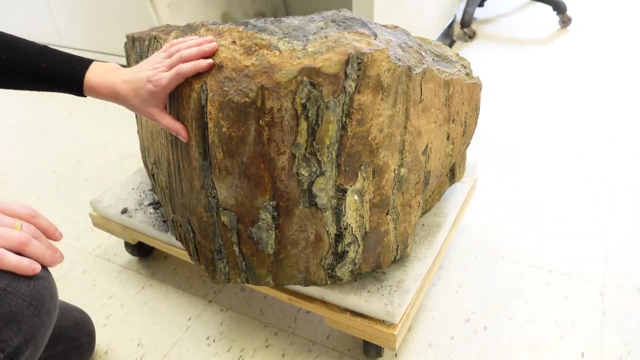 understand better the animals that we're seeing in the fossil record. Okay, so here we have a really cool specimen of a sample from Nova Scotia that comes from the time period that we primarily work on here in the lab, So this is a 310 million-year-old. 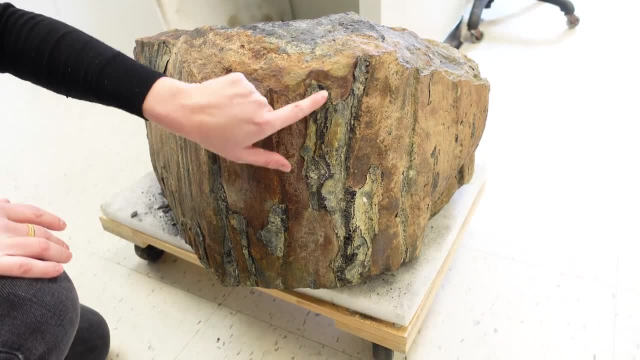 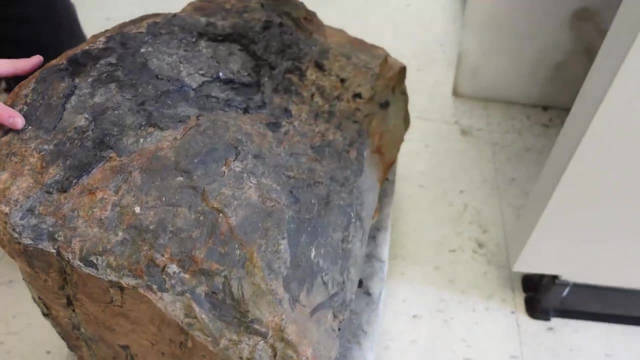 tree stump and you can actually see the pieces of plant material, the carbon, the charcoal on here. But what's really special about these in particular is that during this time sometimes animals fell inside these empty tree stumps and we have the preserved remains of 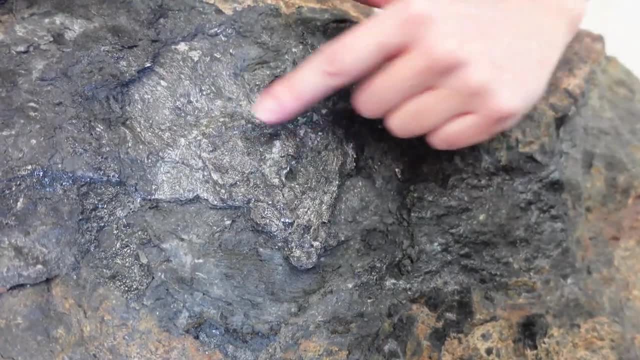 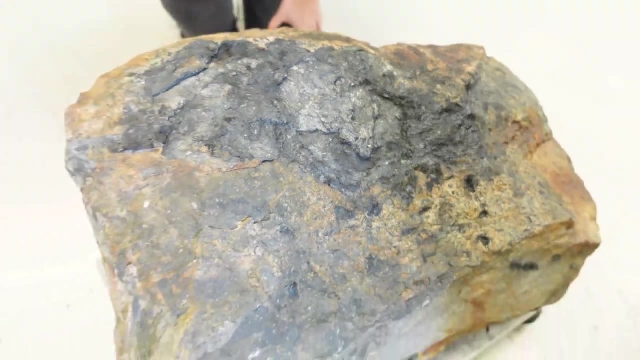 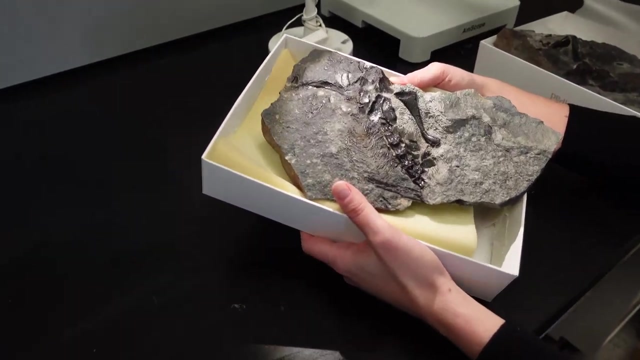 some of the earliest land animals preserved in these. So here's the skull of a tiny little animal that would have been one of our first to walk on land. Okay, so here we are again with another specimen from Nova Scotia, and this is actually a skeleton that was found inside one of those tree. 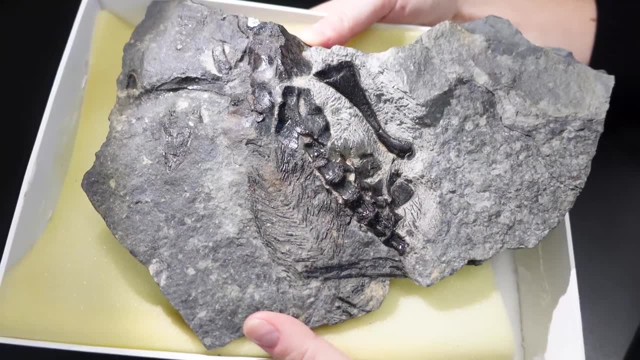 stumps. And what we're looking at here actually, now that we have it all nice and cleaned up in the lab, is we're actually looking at the skeleton of an animal that is more closely related to us than it is to humans. So we're actually looking at the skeleton of an animal that is more closely. 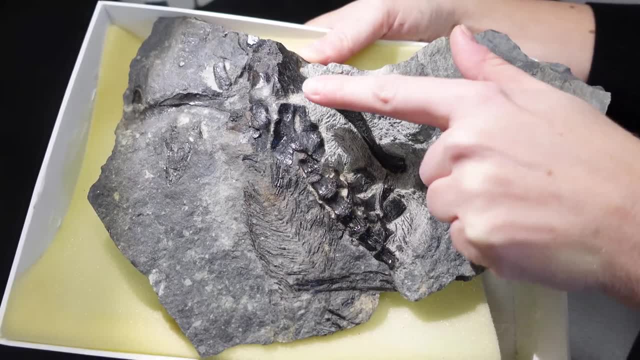 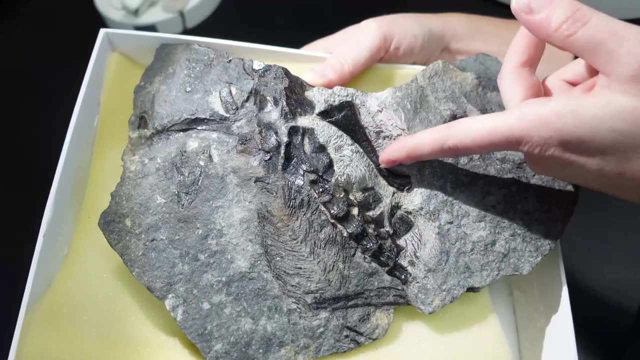 related to us than it is to a reptile, even though it looks a lot like a reptile. So here's the backbone, the vertebral column, your spine and then basically each of your leg bones, the femur, coming out here. 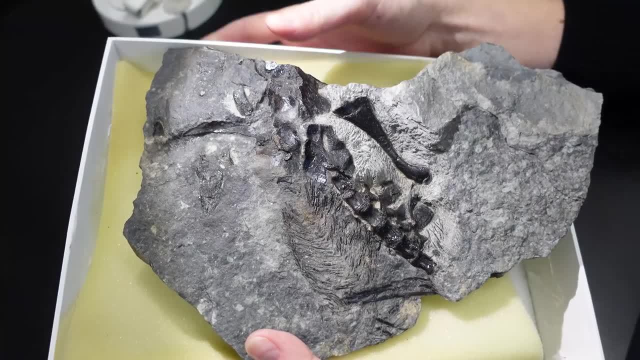 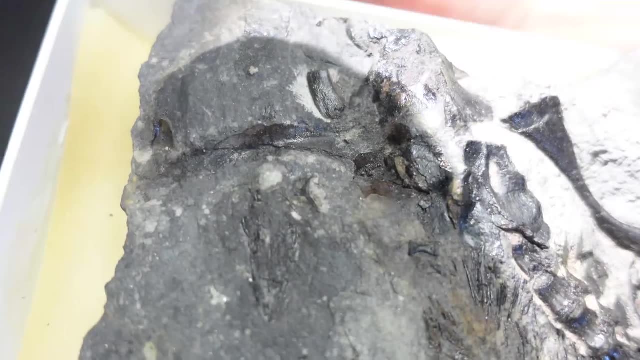 And what was really cool when we discovered this specimen is that alongside this larger animal is the skull of a very tiny individual and there are a few other little isolated bones of this animal, and we identified this as being a juvenile of the same species. 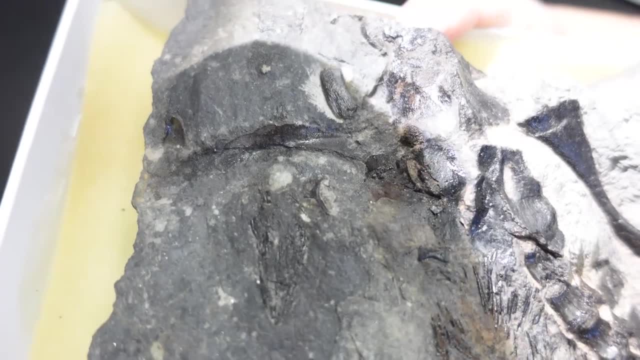 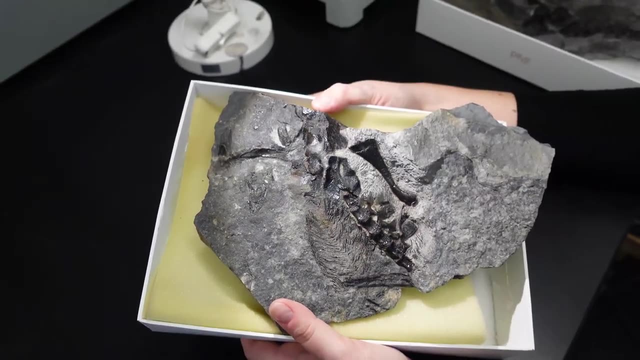 and basically, this is telling us that there is probably a, and this is telling us that there is probably a parent and an offspring occupying this particular tree stump, and this is actually the earliest evidence of a parent animal taking care of its young for a prolonged period of time. 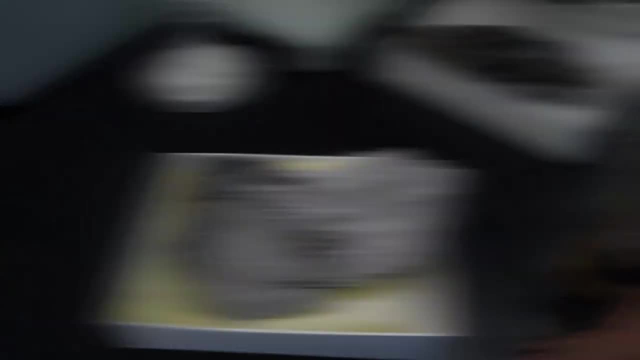 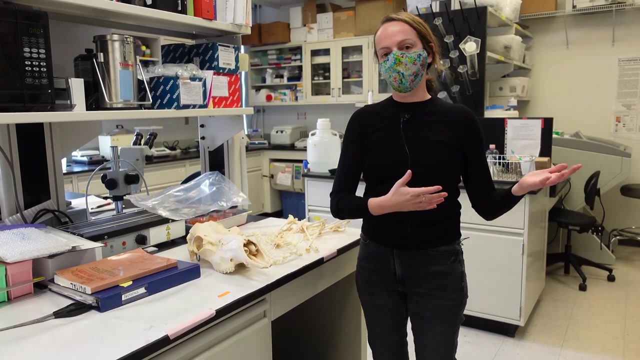 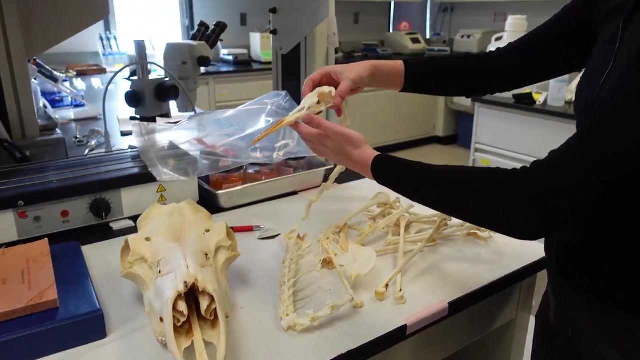 So that was a really cool discovery made out in Nova Scotia. Sometimes in this lab, to understand what we're seeing in the fossil record, we look at some of our modern animals. So here we have the skeleton of a bird and we can actually see the shape of